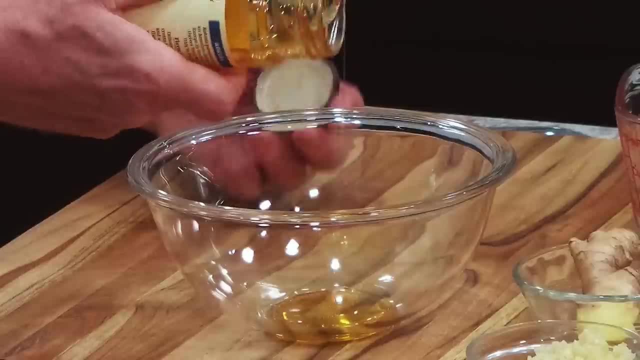 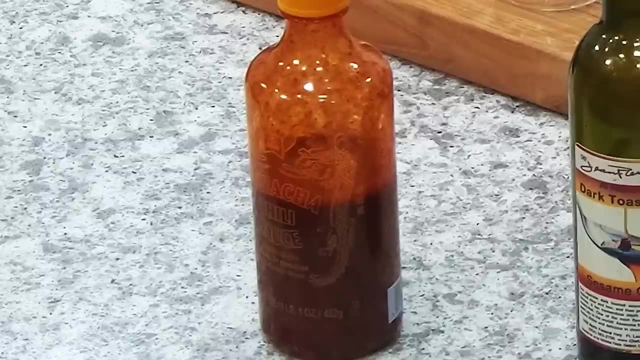 very amazing. Oh well, Anyway, a little bit of honey, And we don't want too much of it, I don't want it to be too sweet- And then we're going to put a little bit of hot sauce. This is going to 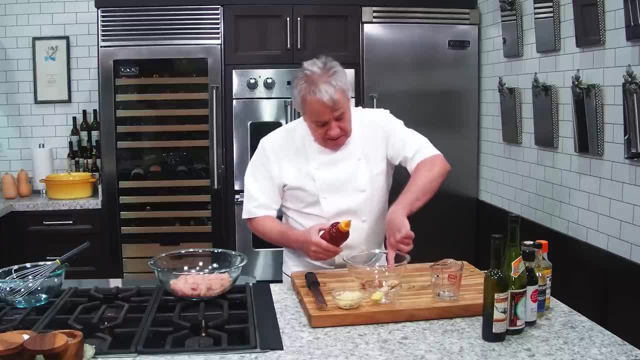 be a little bit of hot sauce. You can put as much or as little as you want. You don't have to put a lot, but it's really up to you. This is you know. there's no right or wrong. Let me get a towel. 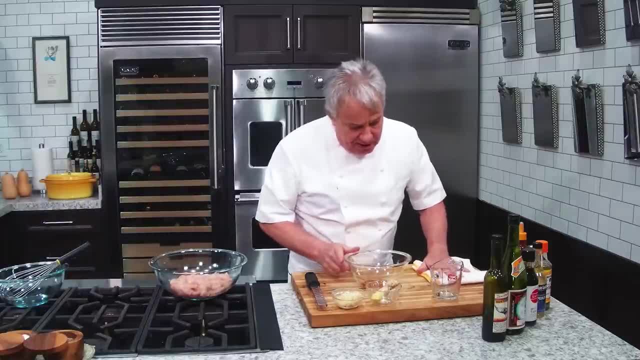 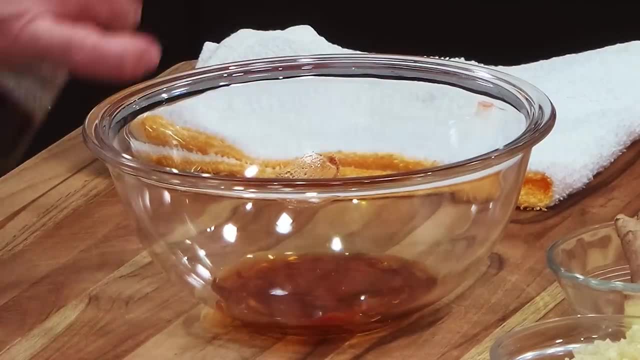 There's no right or wrong here. It's really up to you how much you like to put in. okay, Then we're going to put a little bit of toasted sesame oil in there, Really a little bit of toasted sesame oil. That's going to make it easier to stick on the chicken, And we're going to use a. 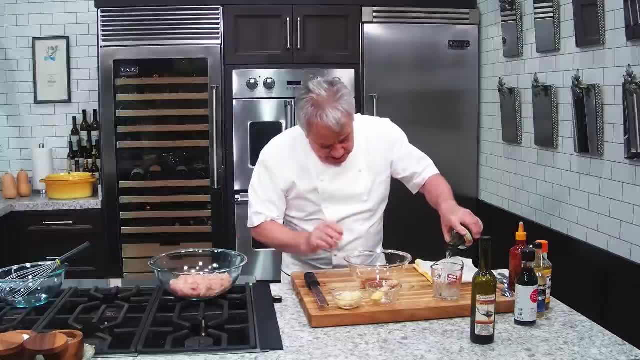 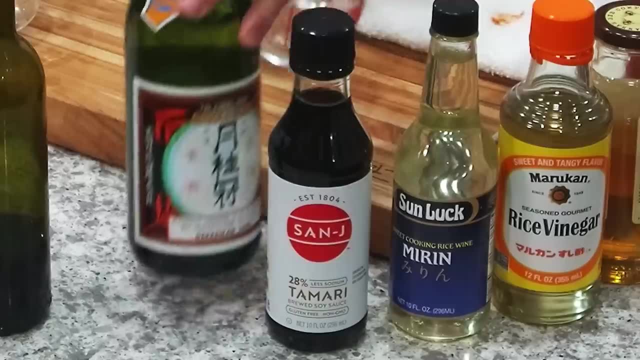 little sake, And I like to measure this, Believe it or not. I'm going to put a half a cup of sake right here. Then I'm also going to put a half a cup of soy sauce. I like to use a tamari soy sauce. 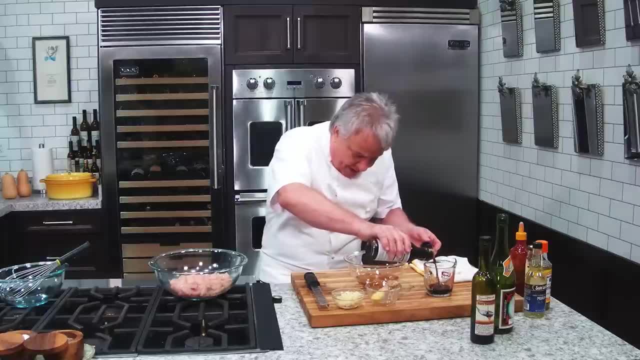 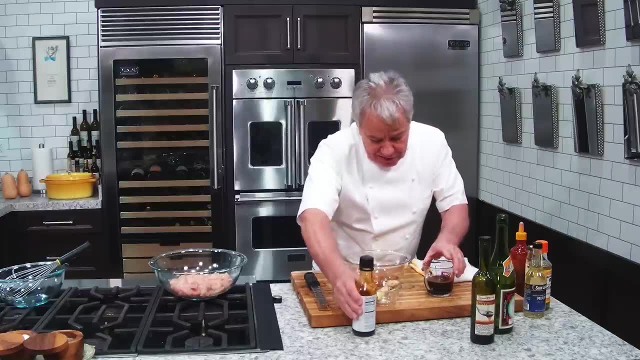 It's naturally brewed. It's better. I like it better. It doesn't have any wheat in it, but it's up to you. We're going to put about the same amount, Believe it or not. you see me measure. I normally don't measure anything, But the good thing is, friends, that marinade. you can use it. 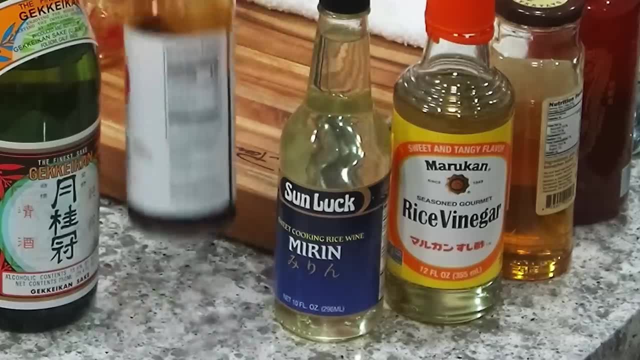 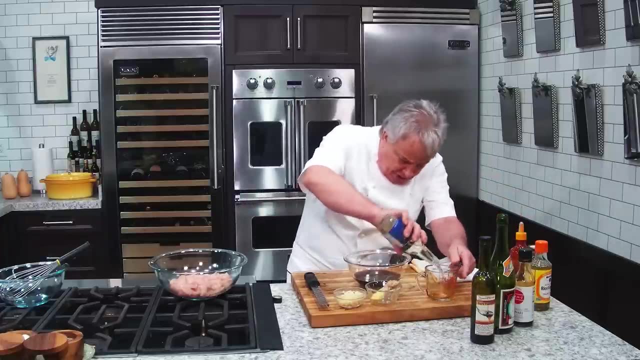 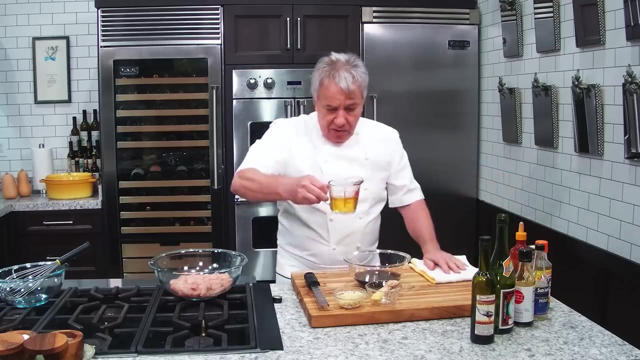 for anything. You can use that for fish, You can use it for all kinds of different things. We're going to use a sweet wine, a sweet Japanese wine. We're going to measure. Look at this, I'm measuring everything. So we're not exactly measuring, you know, just kind of like We're. 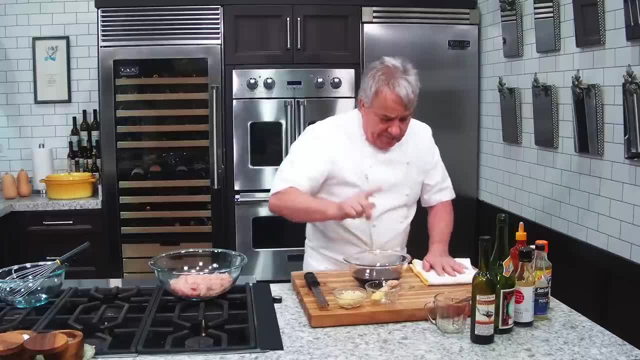 going to do the same thing: A half a cup. I'm going to measure this. Now we got a little honey in there And the honey is going to make it a little sweet, So I like to offset it with a little bit of. 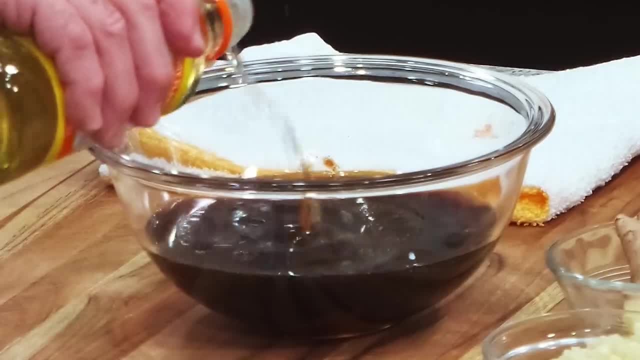 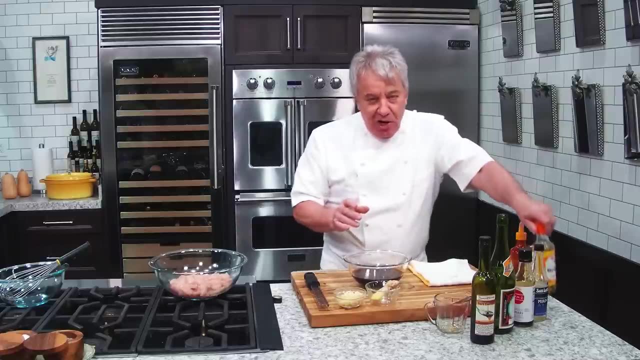 rice wine vinegar. Just a little bit of it, okay, Just to offset the sweetness of the honey and the mirin. so it's not too sweet. There's a perfect balance. In French cuisine we call it gastrique, Sweet and sour, perfectly balanced. So the sweet honey. 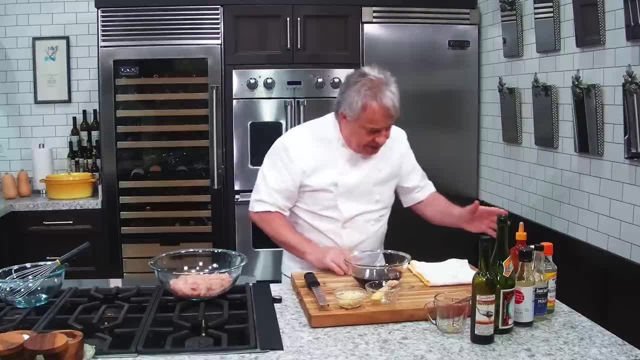 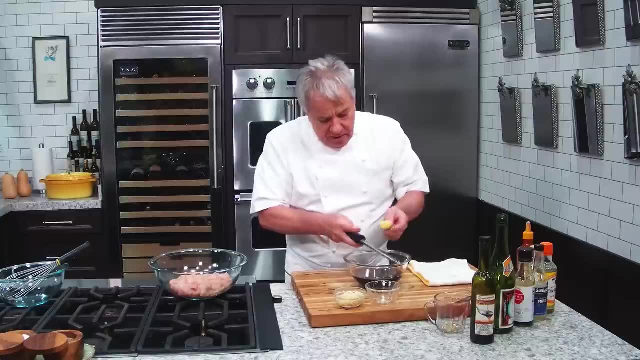 is not too sugary and the vinegar is not acid. Perfect balance, right. So we got everything else. We put everything in there. I hope I didn't forget nothing. Now I'm going to put a little bit of ginger And normally I don't even bother peeling it, But this guy right there needed to be peeled. 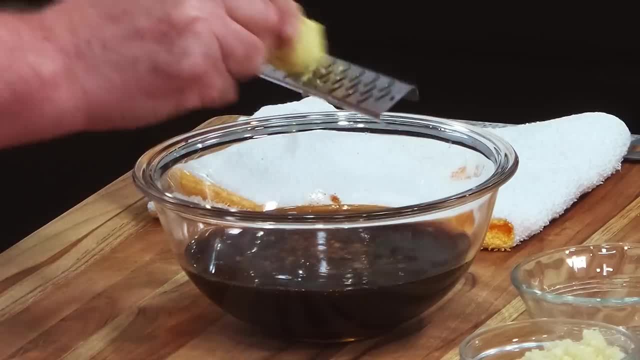 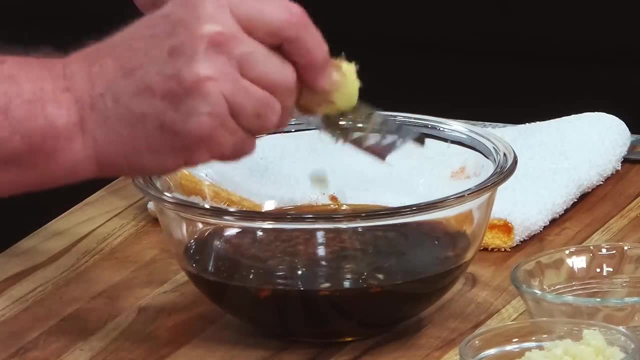 So I peeled it, all right, And I used the microplane grater. Be careful, Careful with these things. Okay, friends, You make pink ginger if you don't be careful, right. And then I have some chopped garlic that we just chopped earlier. Somebody said to me one day he's using the chopped garlic. 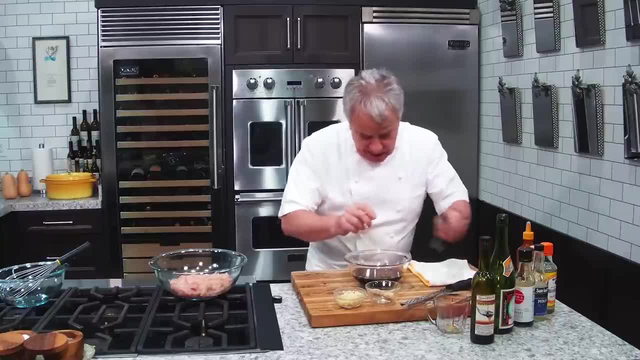 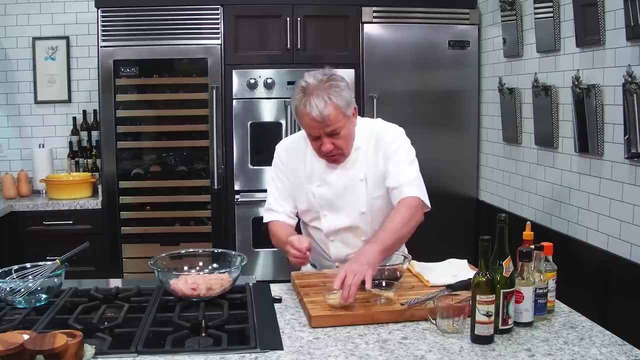 from the store. I would never do that, And so here it is, right there. I just chopped a little garlic. Sometimes I use my garlic puree that a lot of you have been using. So we're not putting any salt, We're not putting any peppers, because obviously we have it right there. We're going to 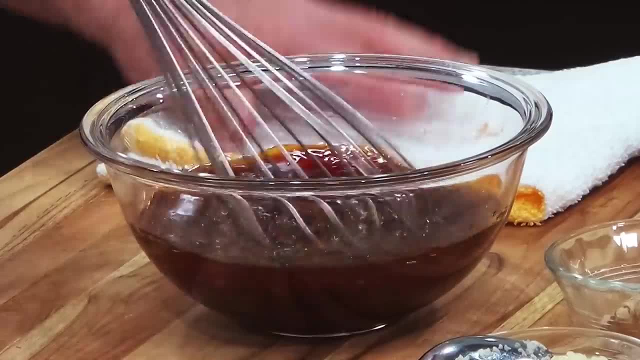 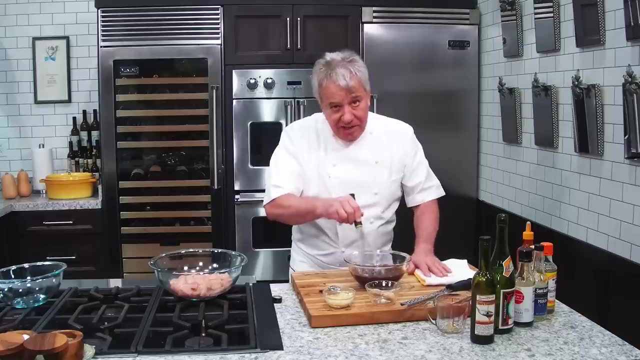 mix this up And then we're going to put it with the chicken. I have a two pound of boneless and skinless chicken breast. Like I said, you can use whatever chicken you like, my friends. You can use the dark meat You can use. some people use a whole piece. 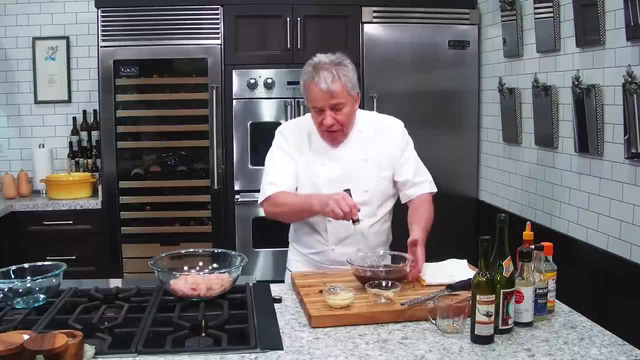 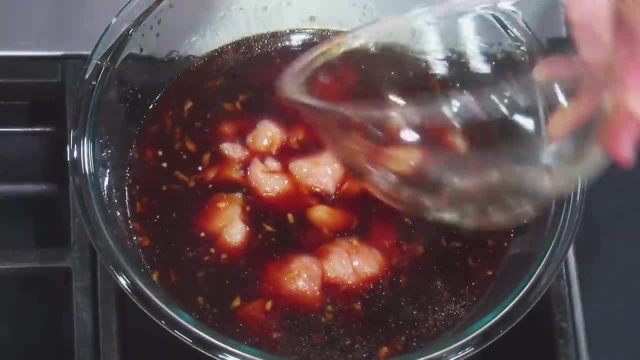 I like to use the bite-sized pieces. We're going to make a stir fry, So it's a mix it up pretty good, And voila, friends. Now all we're going to do, we're going to put this right there, I'm going. 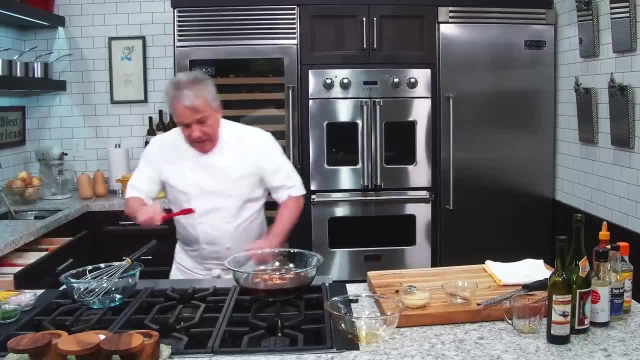 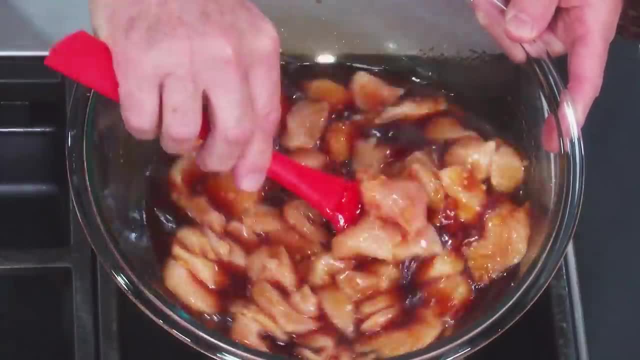 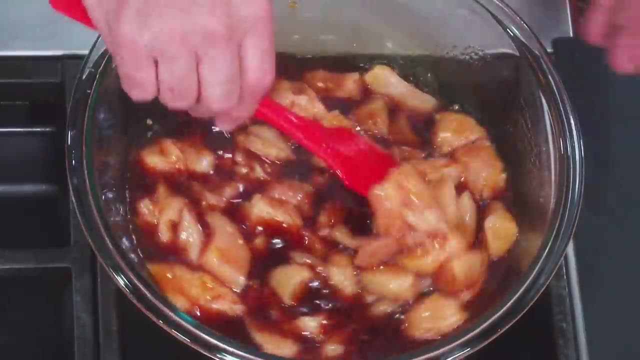 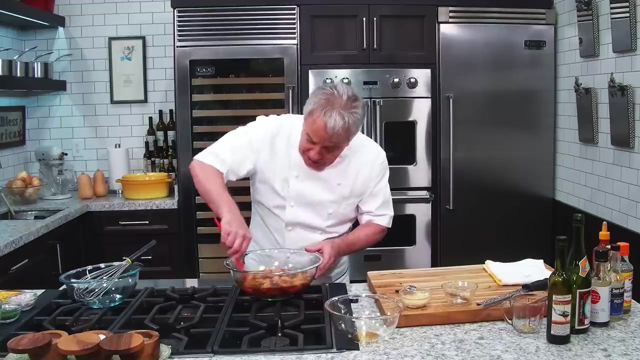 in the refrigerator, friends, for about 30 minutes, minimum 30 minutes. If you can do it 30 minutes, it'll be great And you'll see it's going to be amazing. All right, So we're going to do this, I'm going to put this in the fridge And then, in 30 minutes or 45 minutes, I'm going. 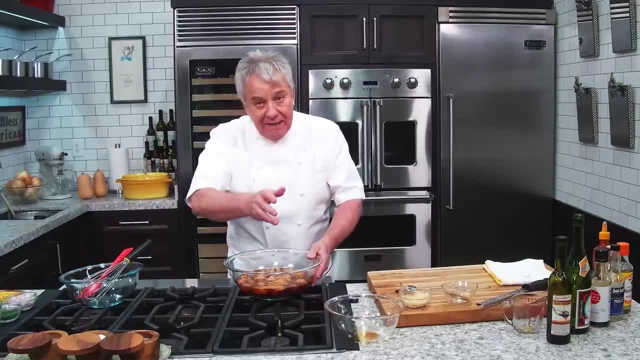 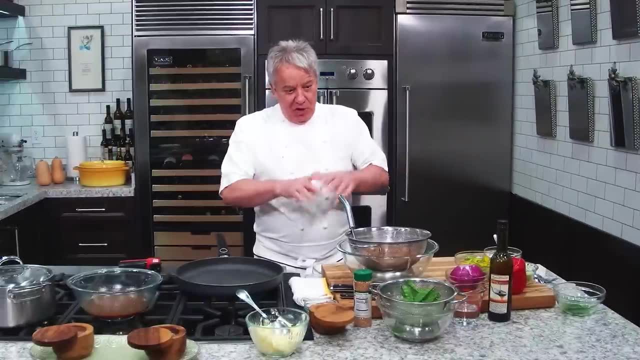 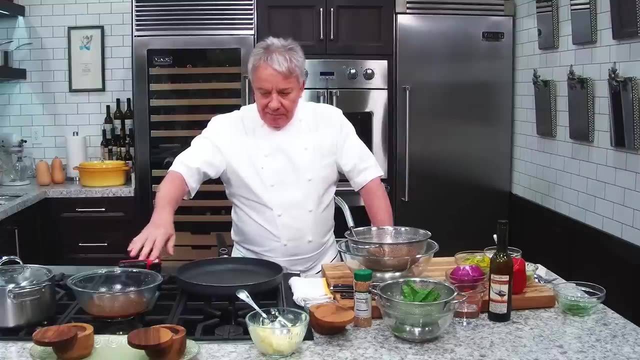 to leave it about 45 minutes. In 45 minutes I'll come back and we'll finish the dish together. Okay, friends, We'll be back in a few minutes. Okay, friends. So what I did is I took the chicken out of the marinade marinade and I drained it. Otherwise it's going. 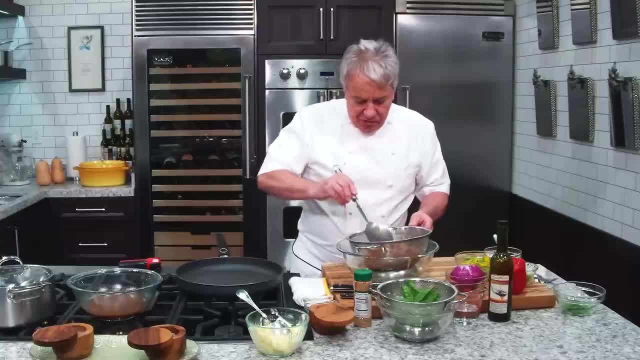 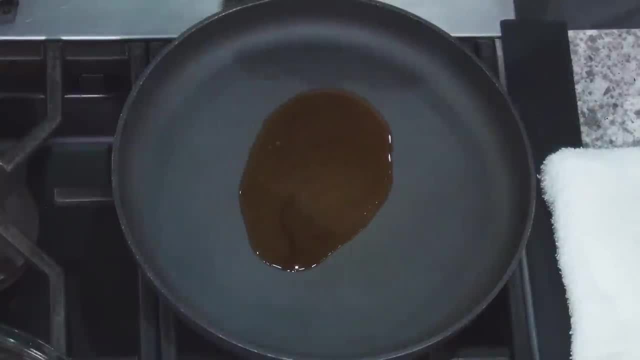 to make a splatter everywhere. Just give it a few minutes to drain, Otherwise you're going to have a huge mess. I'm going to put a little bit of toasted sesame oil. If you don't have any of this, you can use a good olive oil. whatever cooking oil you use, friends, It's really up to you. 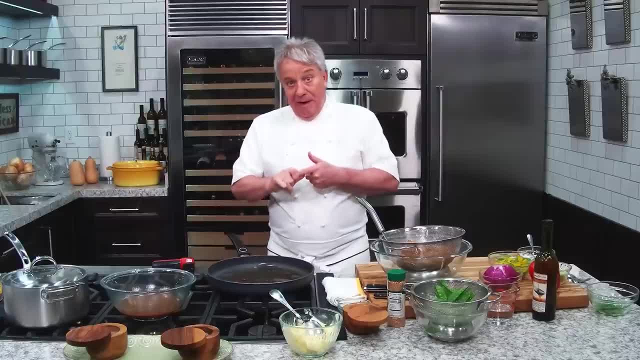 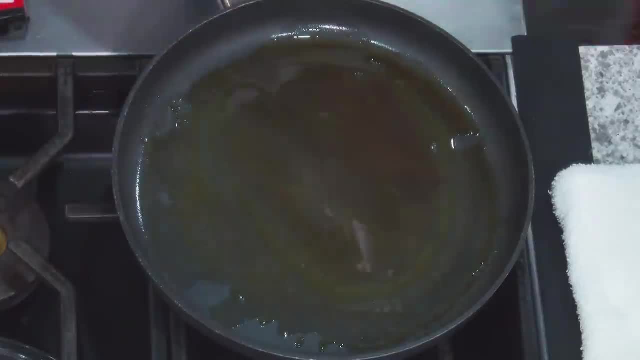 I like to blend that sometime with a little bit of my roasted garlic olive oil. In fact I'm going to put just a little bit, because sometimes toasted sesame oil is a little strong, but I love that flavor. I love that flavor. And then what we're going to do, we're going to put. 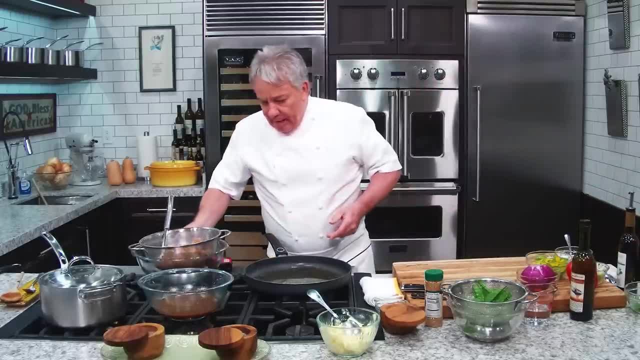 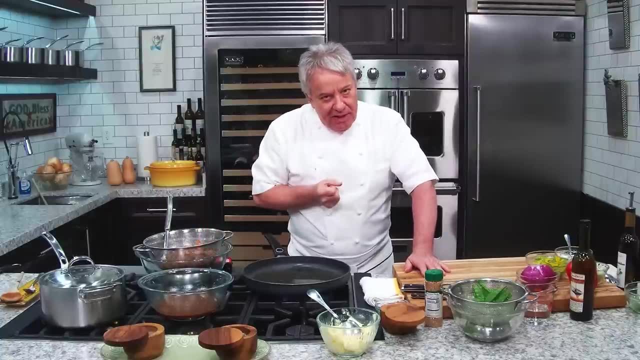 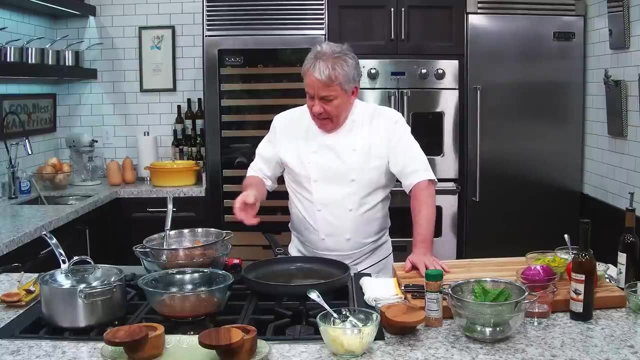 the chicken and we're going to cook it, And then we're going to add the marinade. We're going to add the marinade and we're going to make the sauce with it. I remember this day: one day I was watching the Today Show and they had these Ding Dong guys cooking over there, And he was cooking. 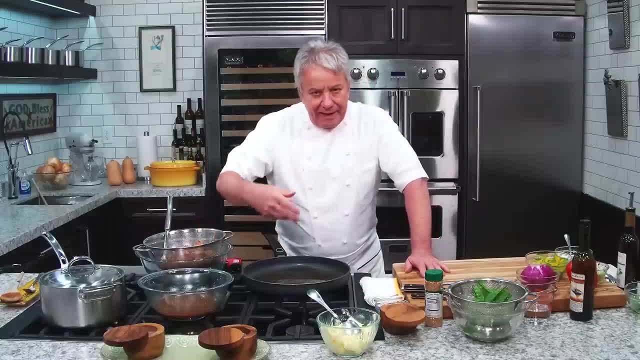 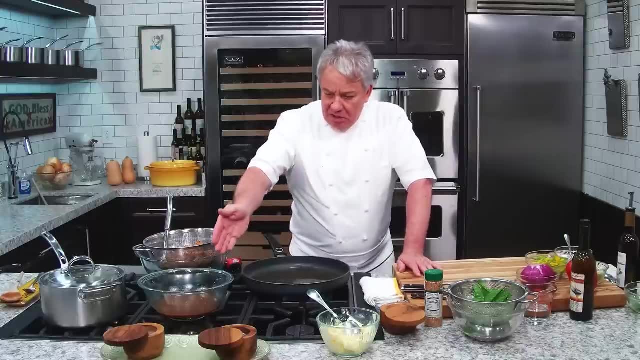 he was marinating a chicken with a little marinade in this, you know, And so he took the chicken out. He said: don't cook the chicken, Make sure you throw the marinade out, He said, because it's full of chicken. It is indeed full. 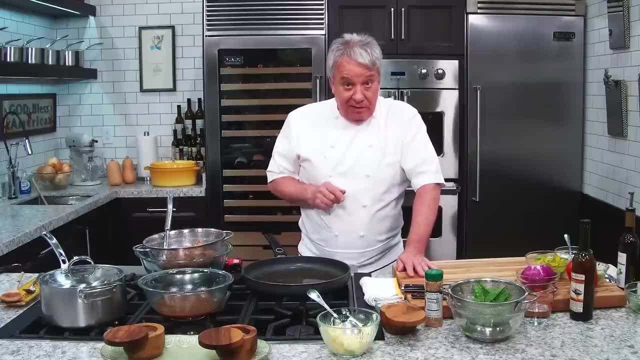 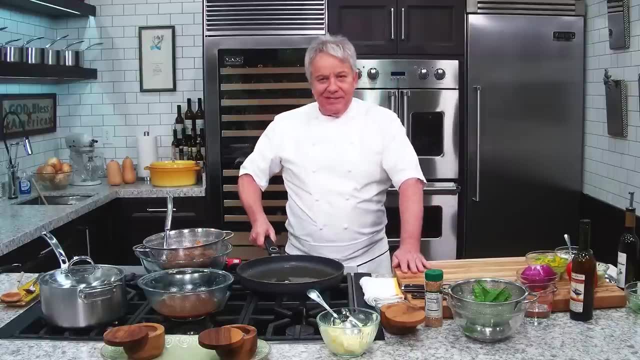 of chicken. He should have thrown the chicken away too. The chicken is full of chicken. Throw that one away. You don't throw it away, you cook it, Okay. So then you're in good shape, All right. So throw the chicken away, All right. So here we go, friends, We're going to put this. 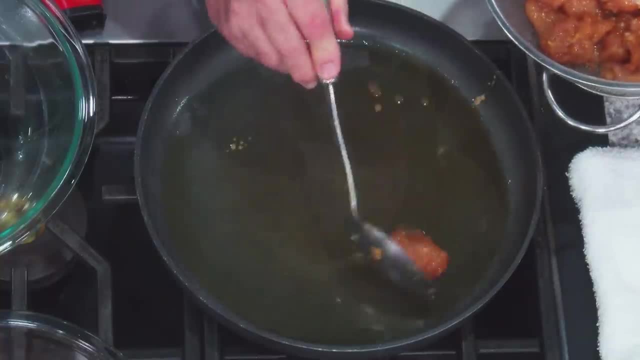 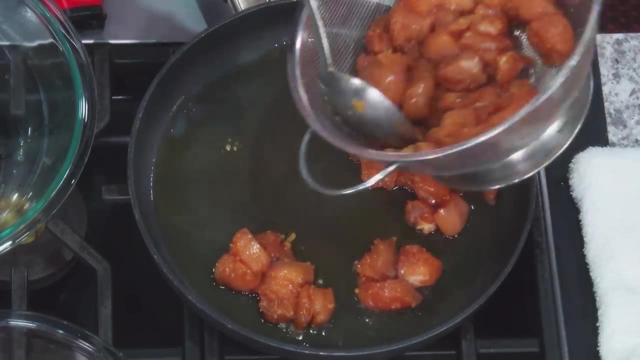 in here. I'm hoping not to get too much plattering. I think we're going to be okay, But it's really important that we do marinate it, friends. It's really really important that we do marinate it, because it's going to be so much better. 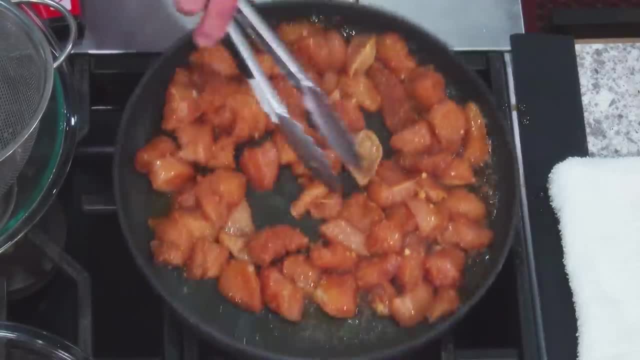 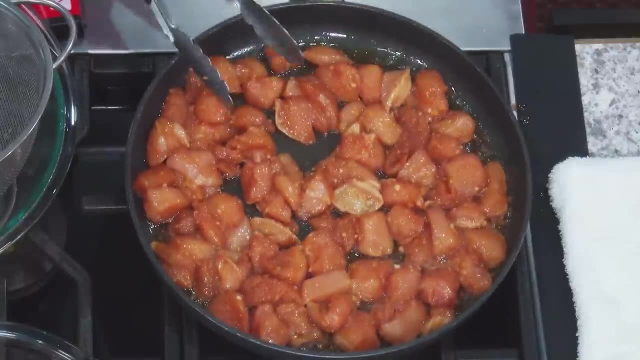 I promise you, So you know what I do, Just in case, I really want to marinate because it's going to be very pretty And I wanted to give it some beautiful color. You see, friends, What I like to do, just in. 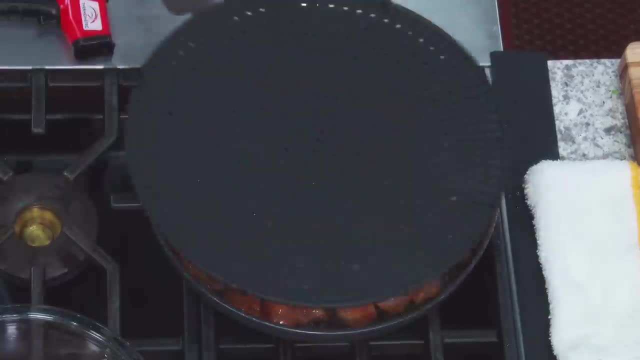 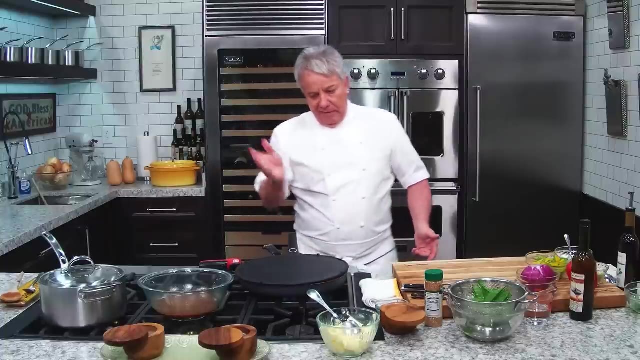 case, I put one of those in there. That's a splatter guard. You can get those at the regular store, regular store, kitchen store, right, You put them out in here and that avoids the store being a, the store, the store being a. 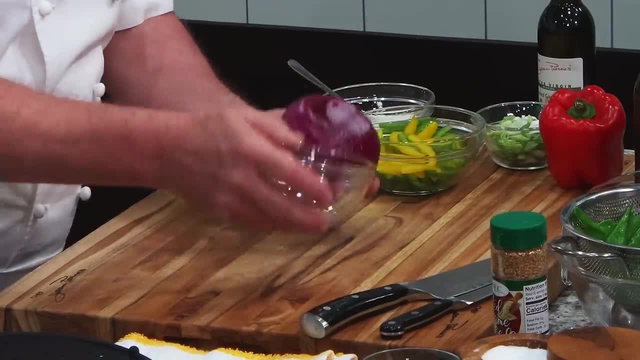 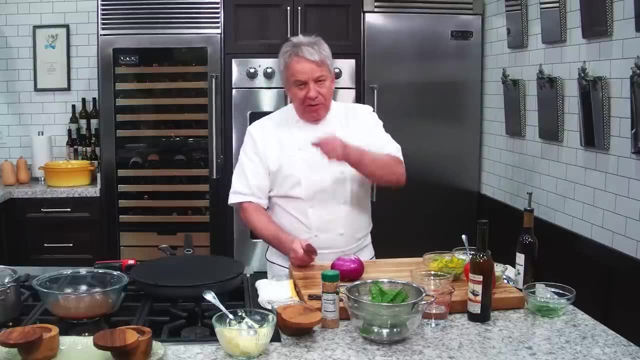 total mess. So, look guys, I never show you how to cut things too much, because I'm doing a video on how to cut all the vegetables, but we're going to put some red onion in there because it doesn't need to cook that long. Red onion you can put on side, you can put it on side side, you can put it. 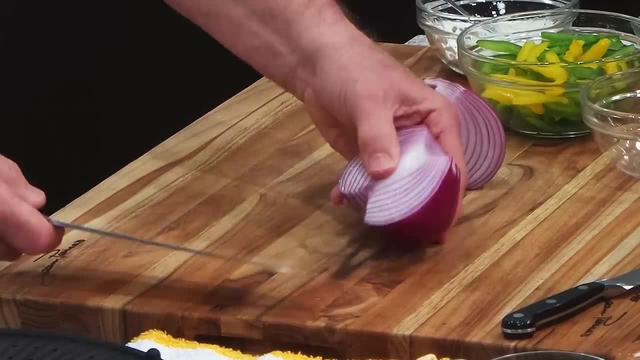 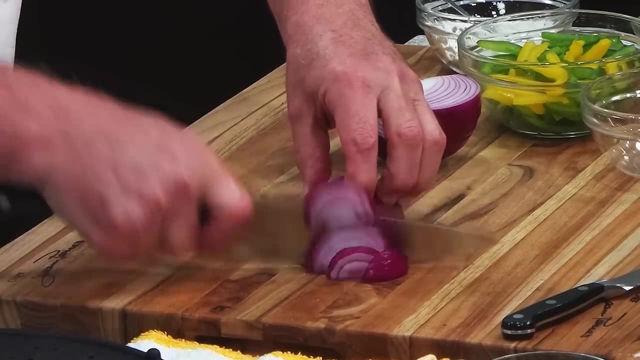 doesn't need to cook that much. So we're going to cut it in half. And remember: when you're cutting onion, friends, Always follow the grain. Don't go against the grain, okay, Unless you're making onion wings And all we're going to do is we're going to cut the very. we're not using a whole onion, We're just. 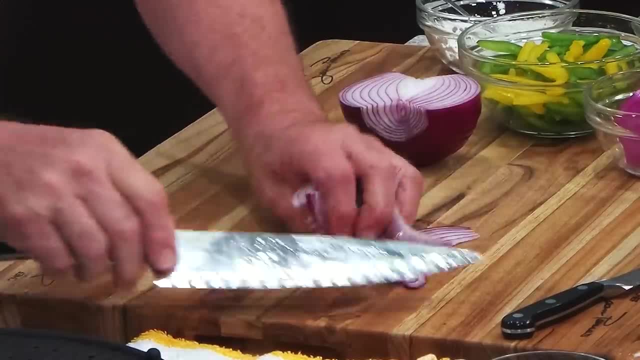 using a little bit. We're just using this, That's it. That's all. I'm using Just a little bit of onion right there, You see, And then we're going to put this in there. I'm only using a little bit. 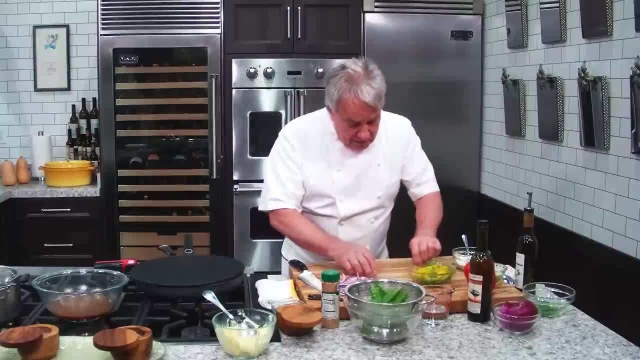 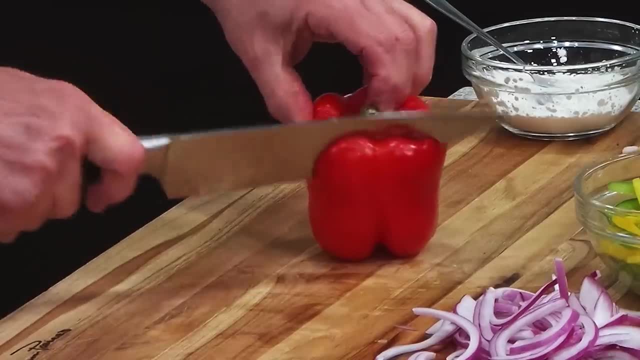 And I cut it fairly thin. you see Very thin, very thin right. Then we're going to put some bell pepper, julienne cut in half, so they're not too long, And same deal here. okay, We're going to take the bell peppers. 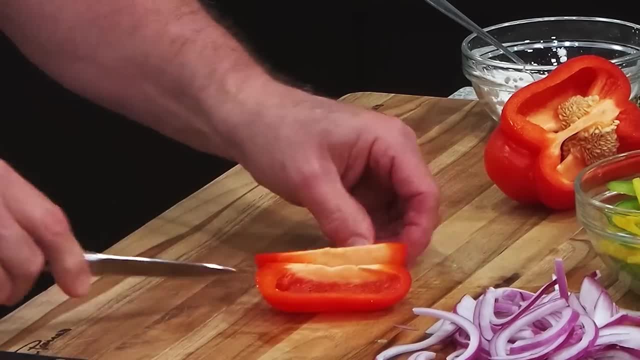 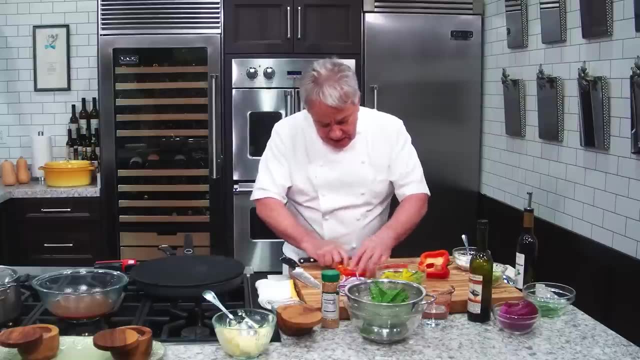 You know, when I cut the bell peppers, friends, I like to cut them like this And I like to get rid of the white. And if you have never tested the white friends, I highly recommend you take a bite out of it And you're. 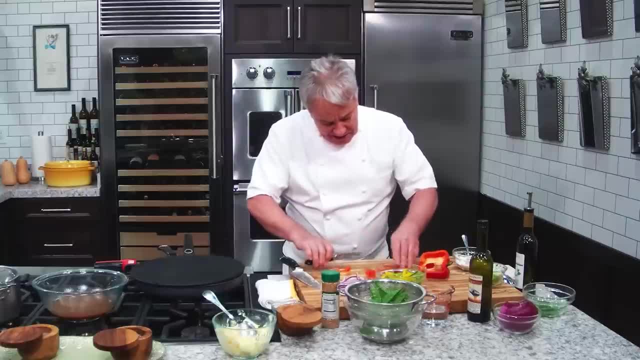 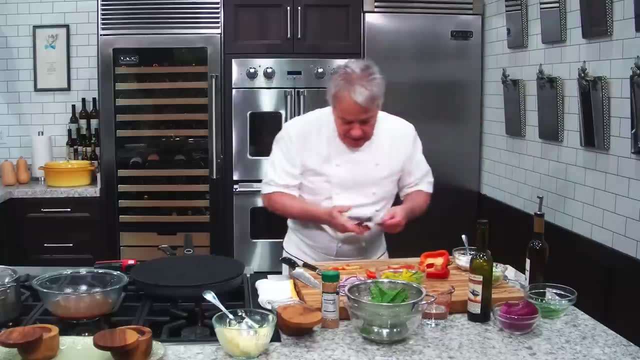 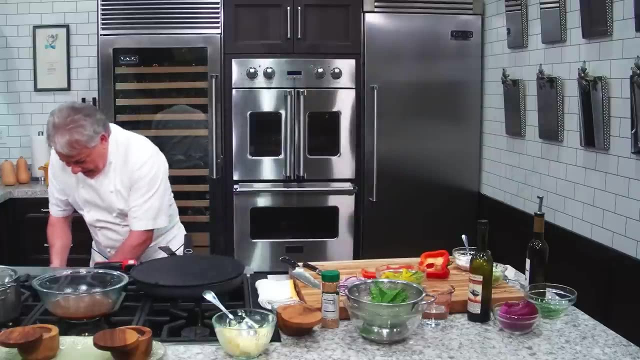 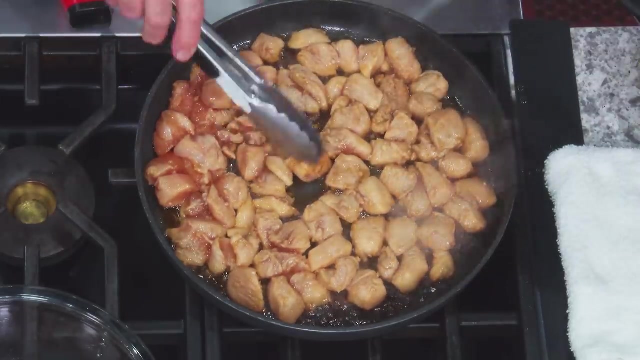 going to be amazed at how not so good it tastes like. Plus, it's got terrible texture. So we get rid of this. We put this in our garbage, Get rid of all the seeds also, And we better check our chicken. You see how it's doing. How is it doing over there? How you doing, buddy? Let me check on my tongue. Let's see how we're. 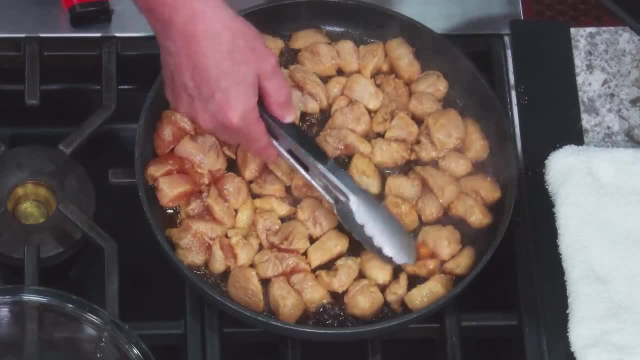 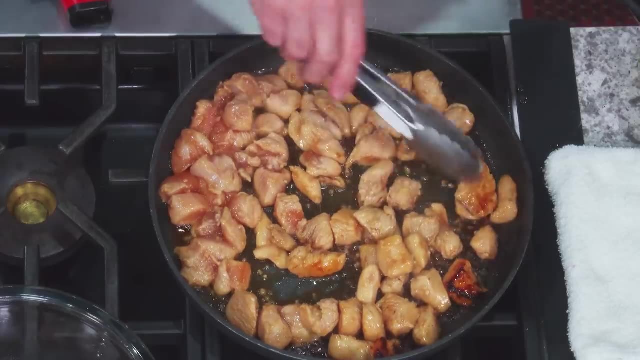 doing. What are we doing? We're doing, we're doing. Yes, that's what I want, right there, Give me some color, There you go. That's what I want. Why is it only over there? Mamma mia, You see, that's what I. 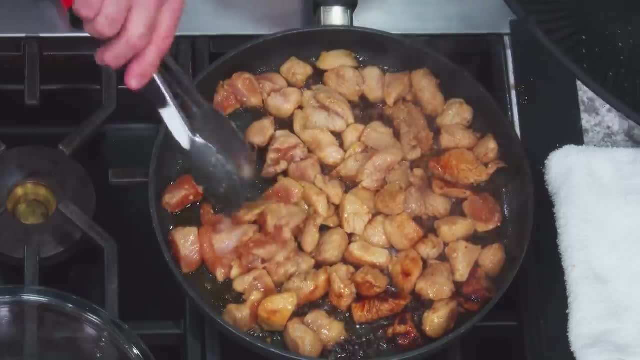 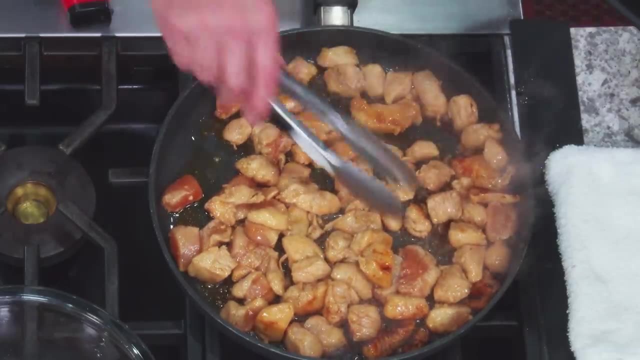 want. right there, friends, Beautiful color. Look at this, Mamma mia, Let's put everything on that side. eh, The other side Doesn't give me as good color. Look at this. We mix them up so they all look good. What do you? 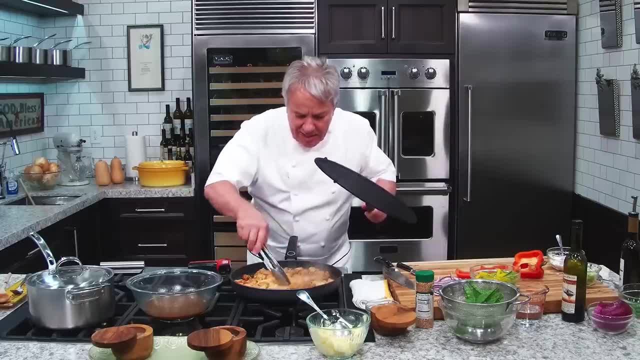 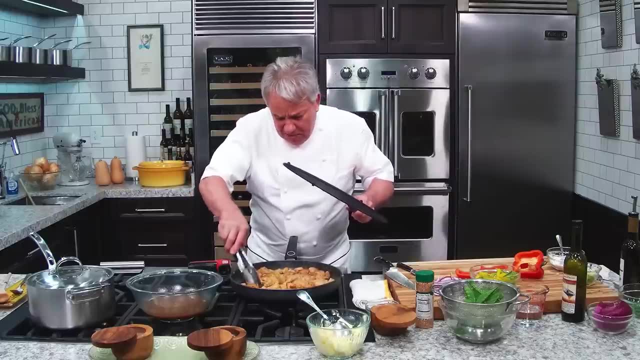 think. You see, that's what I want, That's why I did all the marinade thing, And then we're going to put the onion in there- Red onion. We're going to put them first because we like to put the onion first. 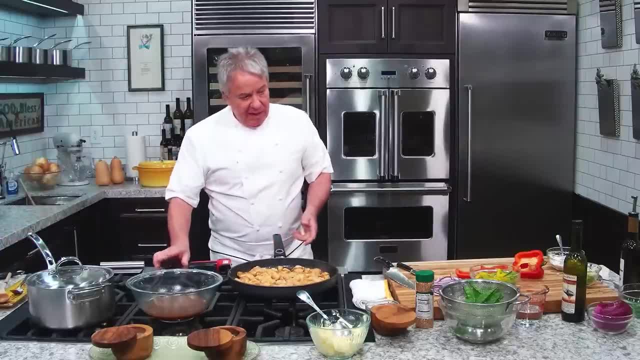 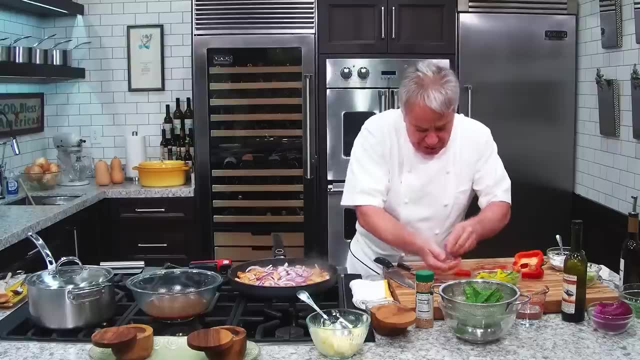 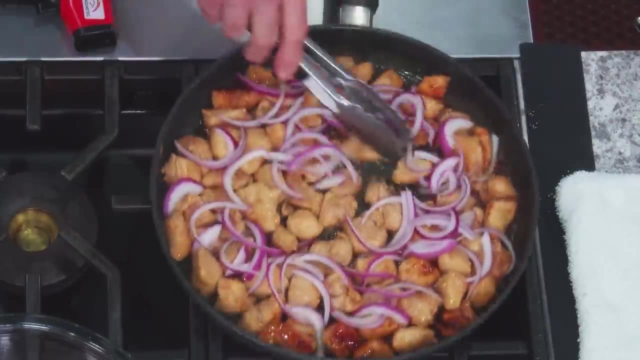 That did pretty good. actually, It didn't splatter that much. right, It didn't splatter that much because I, uh, I, um, I grain, I got rid of the, uh, some of the juice, And then we're going to put it back in. You'll see, This is very cool, friends, Saute a little uh onion in there. 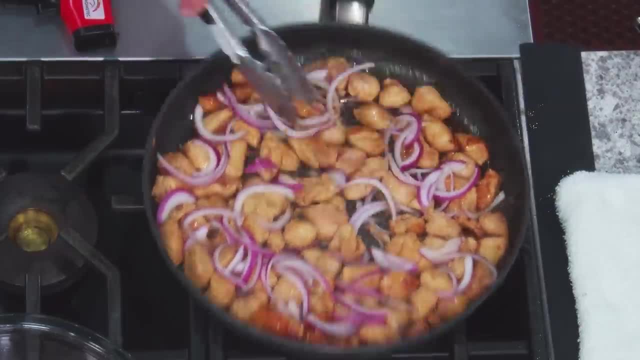 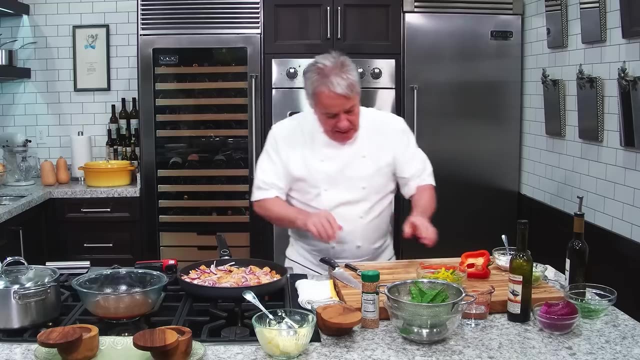 Remember red onion. They don't need to cook that long. That's why I put them in there. Plus, they look kind of cool, right? Bell peppers- What do we do with this? What do we do with this? I'll tell you what we do with this. Remember, friends, when you're. 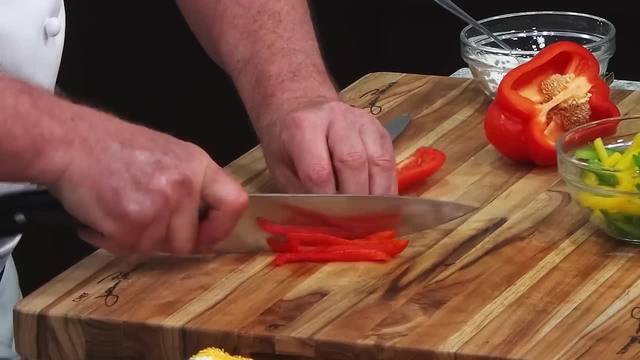 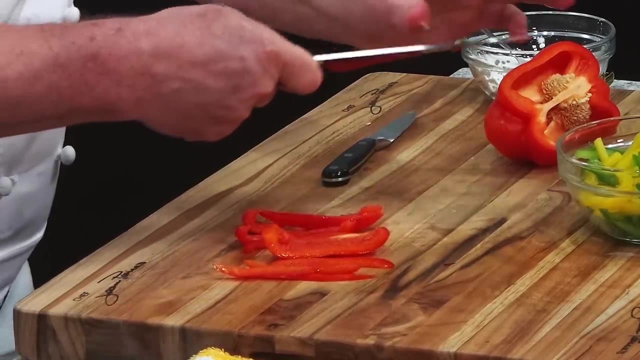 cutting bell peppers. always make sure you cut the bell pepper skin side down, Skin side down, not up, okay. And when you use your knife, mamma mia, look at, I got seed here. Always this way, remember This way. 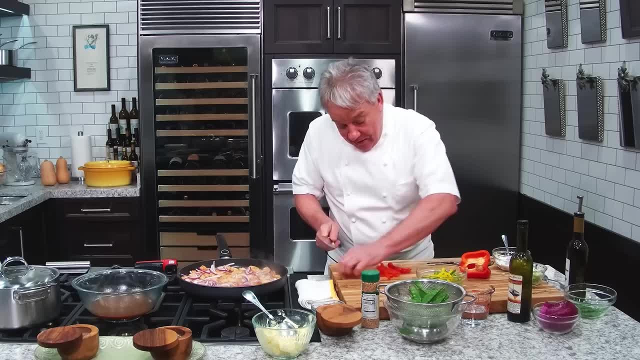 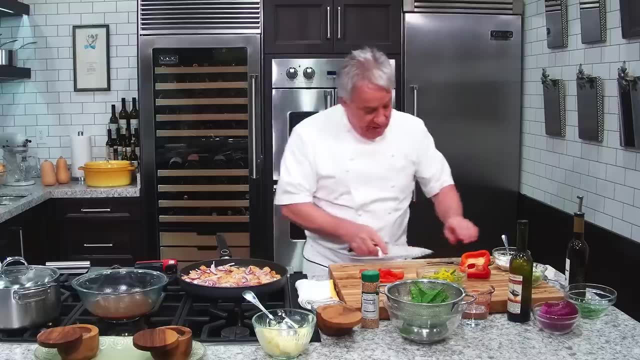 This is how you use a knife correctly. We do it. I know there's so many media. I want to do friends, Like you see, And then I cut them in half. So I got small julienne, all right, And we're going to put all this. 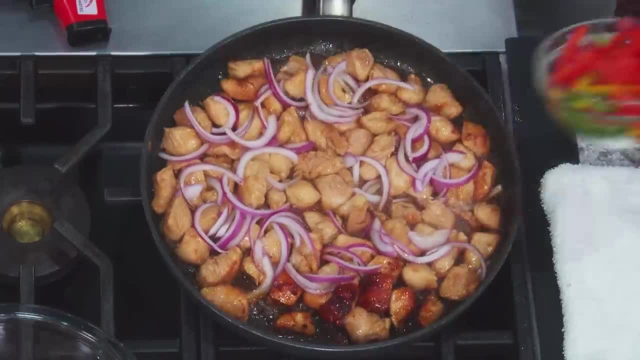 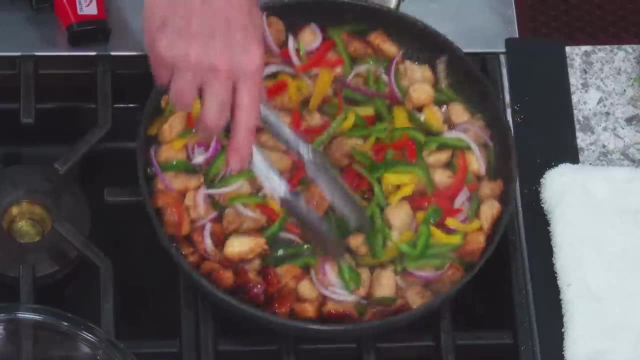 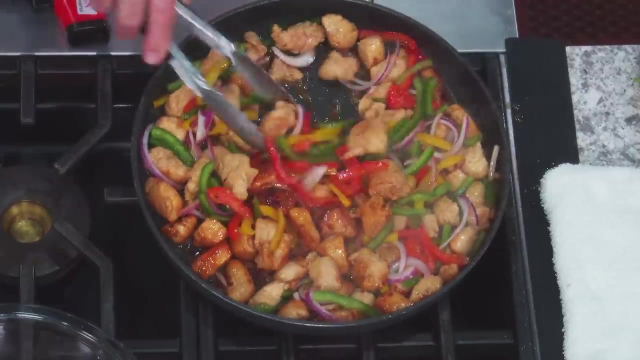 in there. now We're going to put it all in there, friends, All in there, Just like this. That doesn't need to cook, Not long. you see, Going to saute a little bit longer, And then we're going to put our marinade. Look at this. 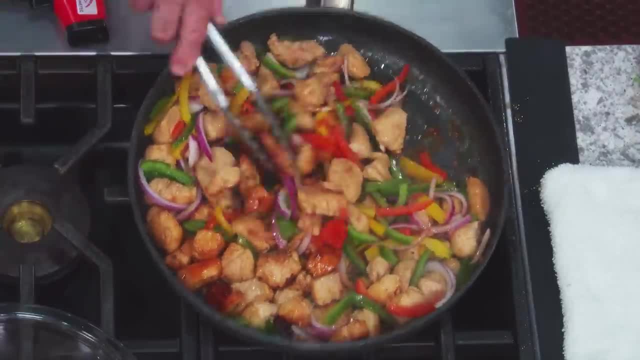 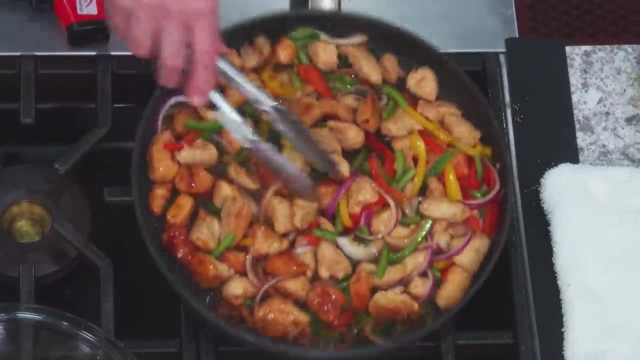 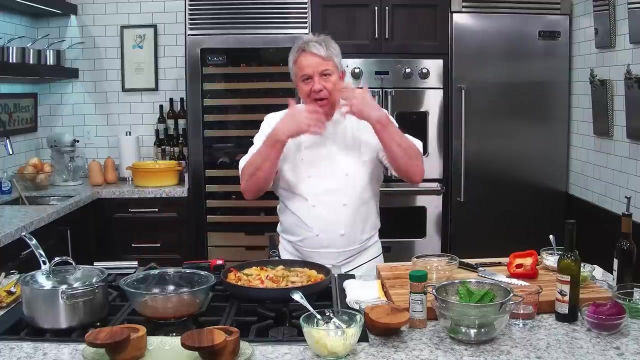 This is beautiful. That chicken is looking good. Yes, sirree, Let it cook. See, It looks pretty, doesn't it? It's very important. It's very important to look good. Then I got the snap peas right there, friends. 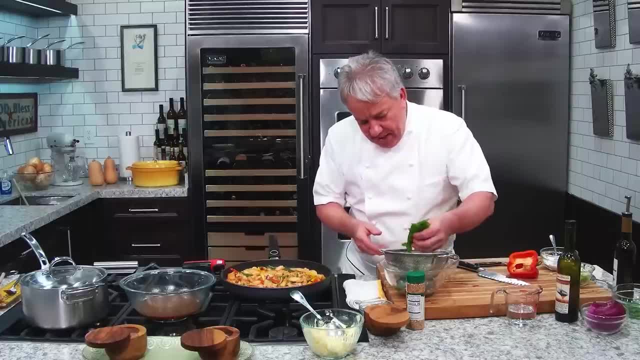 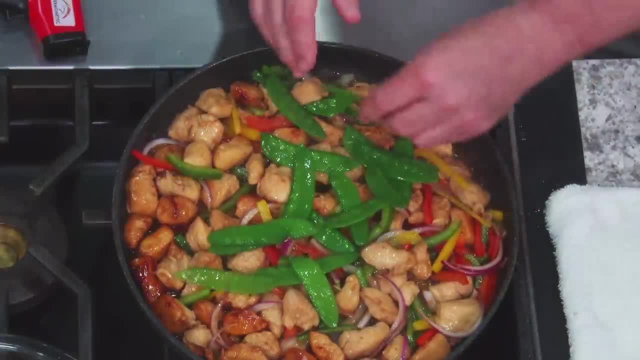 And we're going to put them. snow peas, snow peas, We're going to put them on there. I poached them really quick in boiling water for a few seconds And we're just going to put a few of them in there like this: You could put the broccolini, You could put broccoli, You can put some people put spinach. 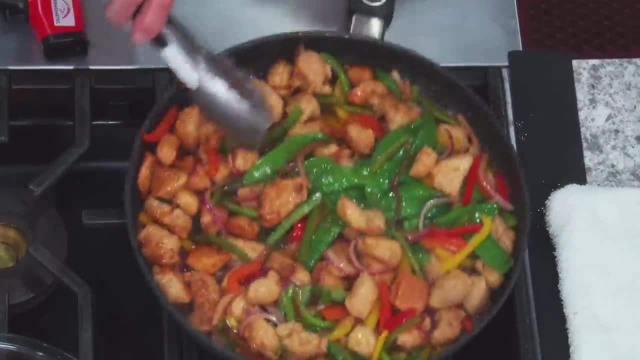 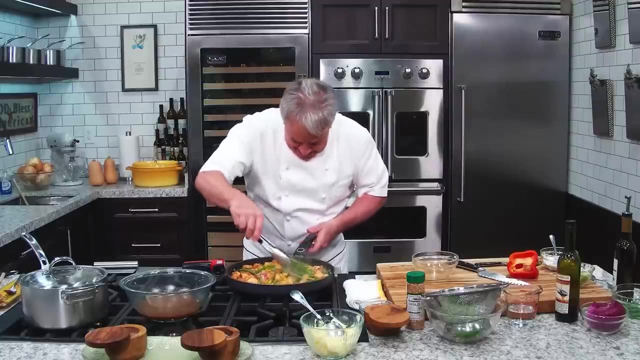 in there. I just love a few little vegetables Right here, my friend. Look at it. Look at that Gorgeous. You haven't seen nothing yet. I love my life. I got the best job in the world, don't I? 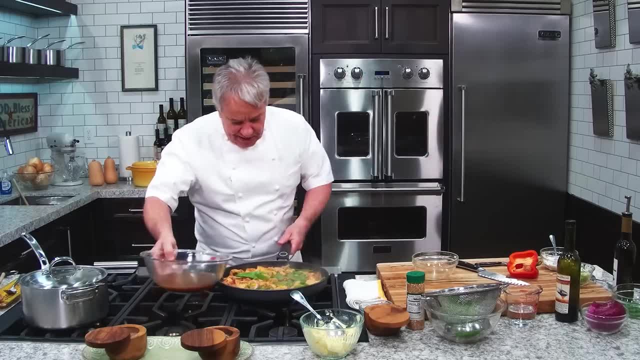 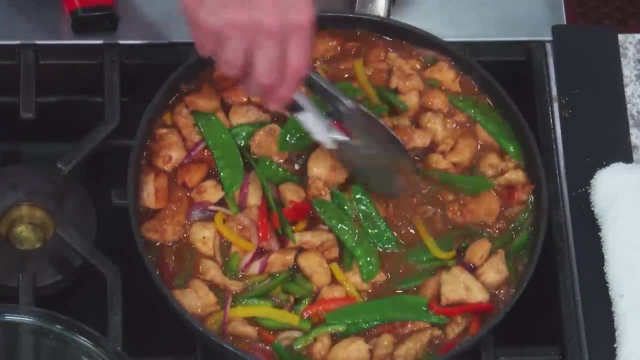 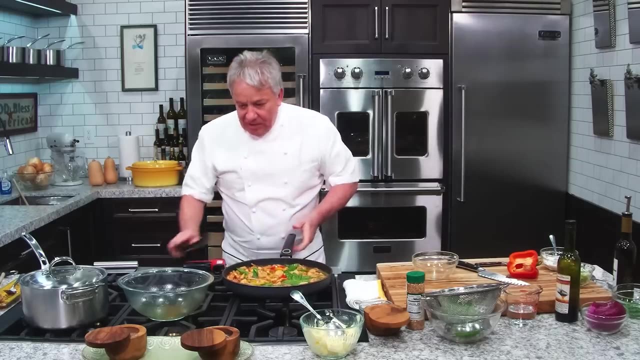 I love to eat and I'm making food for a living. Look at this, friends. Look at this. Yes, sirree, Yes, sirree, Bob, That's an expression, isn't it? So look, friends. What's wrong with this picture? 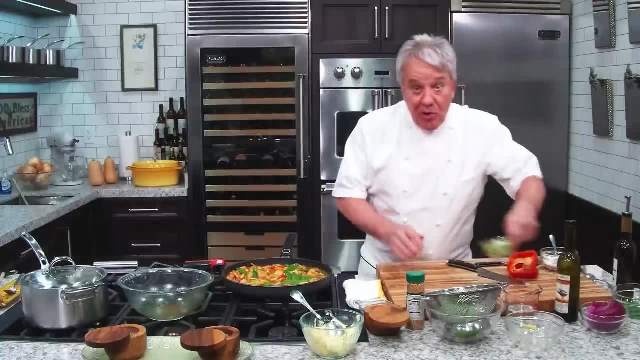 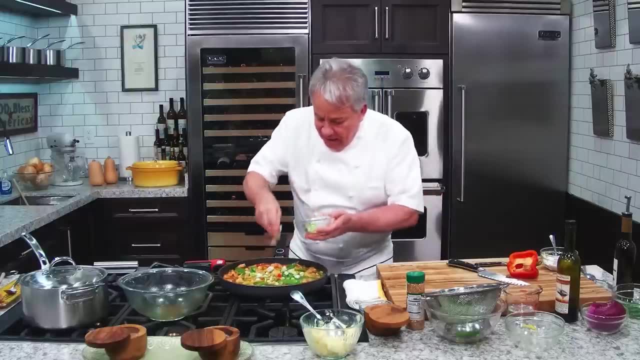 You know what's wrong with this picture, right? Yeah, let's put some green onion, Green onion, We got a lot of stuff in there You can skip. if you don't have one of them, You don't have the peas. 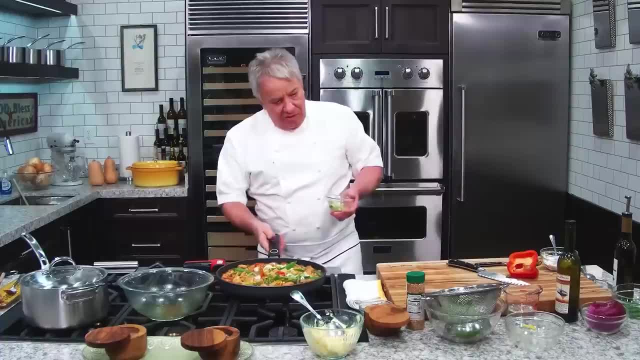 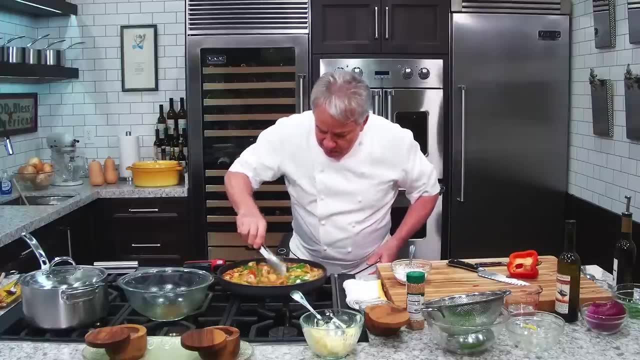 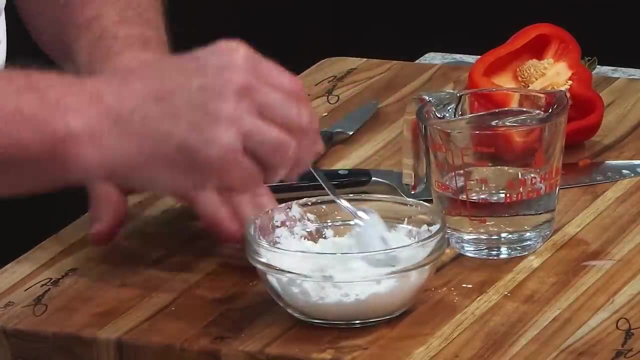 You don't have the green onion, Don't worry about it, It's still going to be very good. Okay, we're finishing cooking the chicken And now we're going to transform the texture of all this, Make it look real pretty. We're going to put cornstarch- All right, We could dilute it in sake. We could dilute. 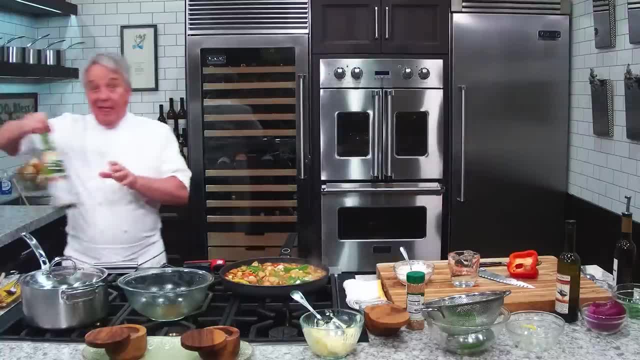 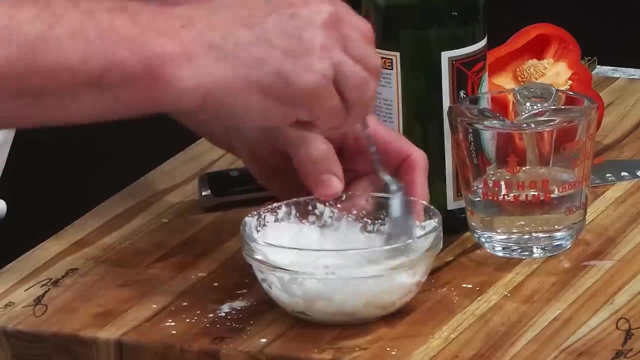 it in. hey, why don't we dilute it in sake? I like that idea. Dilute it in sake, Here we go, Here we go, And then we're going to make a cornstarch slurry With this, And then we're going to add it to it to give it a beautiful texture. my friends, 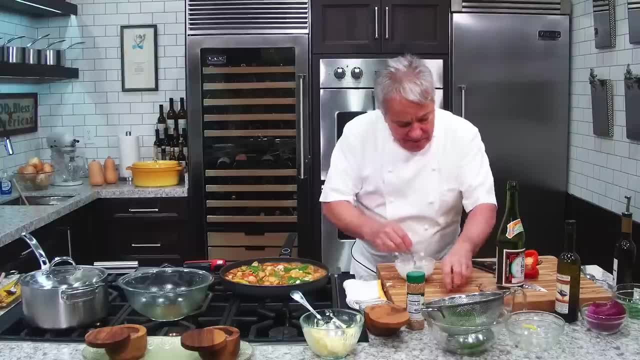 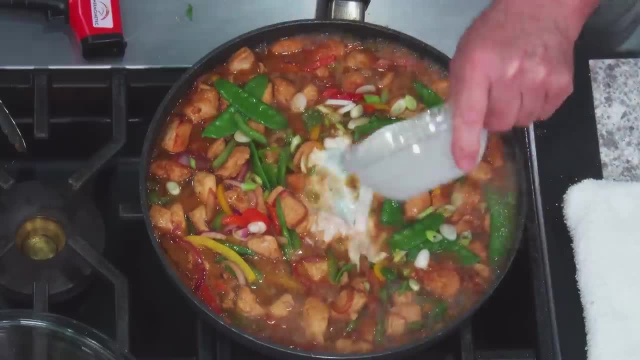 So it's okay if I add a little extra. You can do, dilute it in water. I have the water ready. But why use the water when you can use sake? Since it goes with the recipe, friends, right, Take it, Put a little bit first. okay, Don't put too much, because if you put too much, 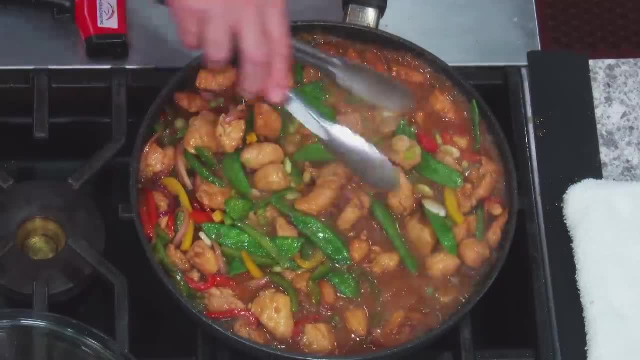 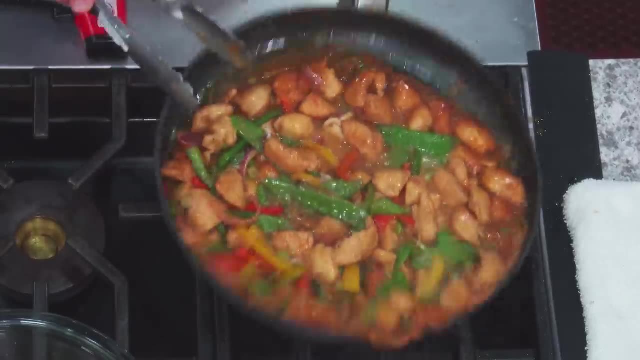 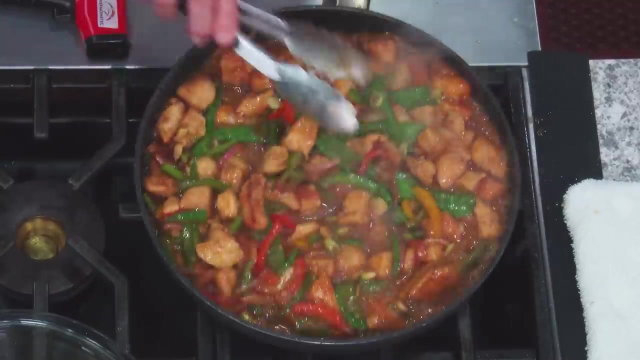 then you'll have too much. I'm telling you, tonight I'm a philosopher, This afternoon I'm a philosopher. friends, There you go. It's looking beautiful And now we know our chicken is cooked. You see, We know our chicken is cooked, friends. 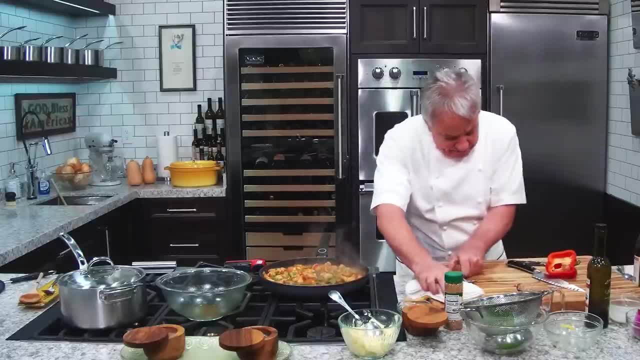 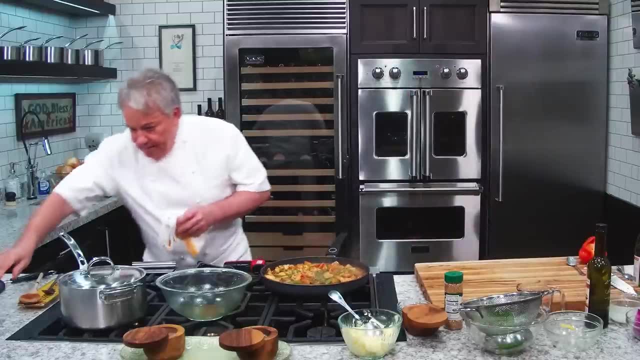 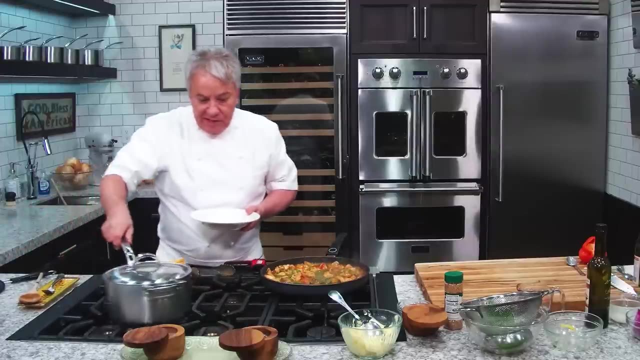 And we have it right there, Beautiful. So now, all we have to do, friends, at this point, is get ourselves a serving plate, And I got beautiful rice right here. Matter of fact, we made a video on this, friends: how to cook the perfect rice. 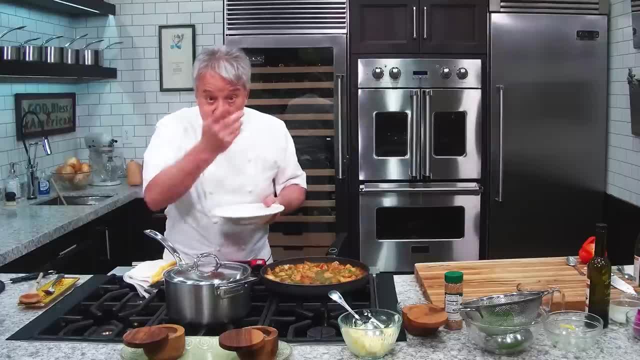 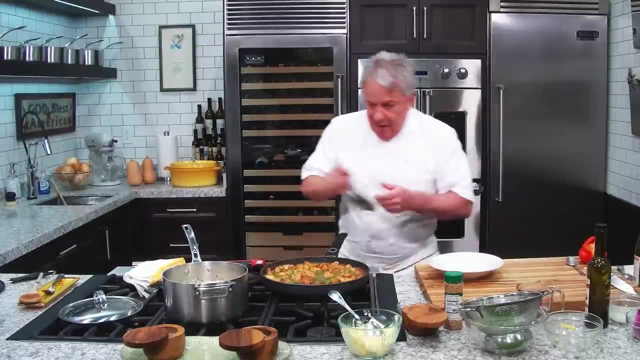 If you don't have a rice cooker right over there, make sure you check it out. We released it a few days ago. I believe We got the beautiful rice. Let's get it panned. Let's get a fry pan right there. Let's put the rice to the bottom. 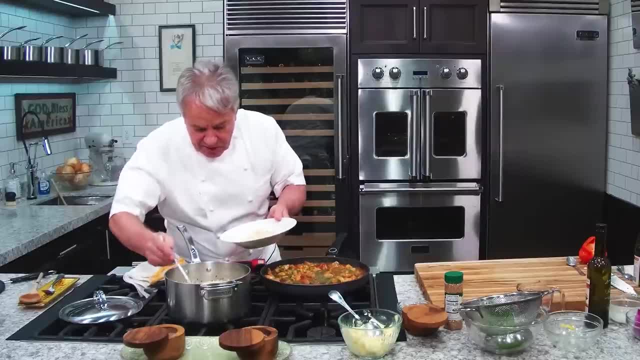 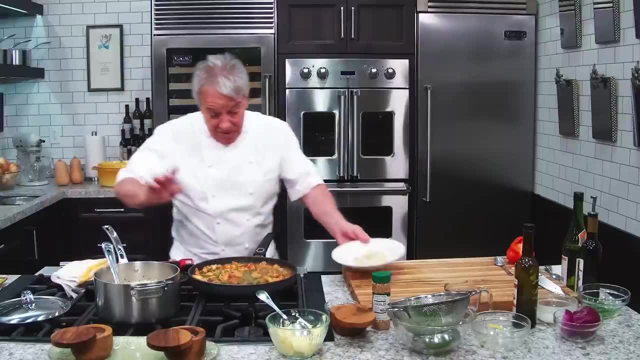 Look at it. Rice is beautiful. eh, Rice is gorgeous. friends, Look at this. This is how to cook perfect rice. You got to watch that video. if you haven't watched it, friends, It's wonderful. Let's put the. 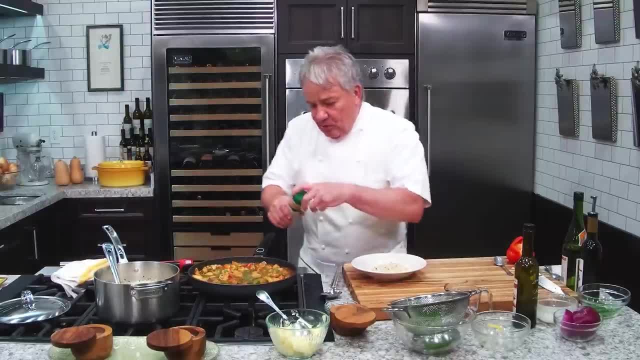 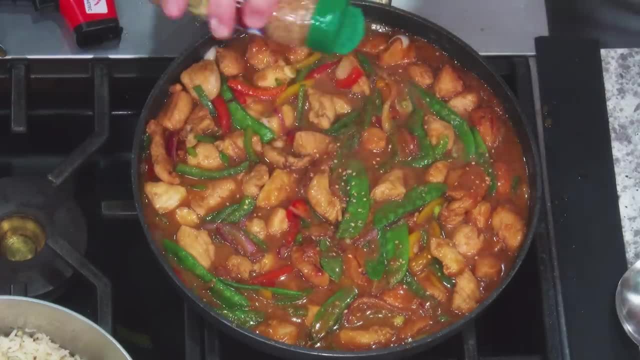 the chicken in there. friends, And you know the last minute what I like to do. I like to add a little bit of toasted. How do you open up this thing? Toasted sesame seed. You can use the regular sesame seed.